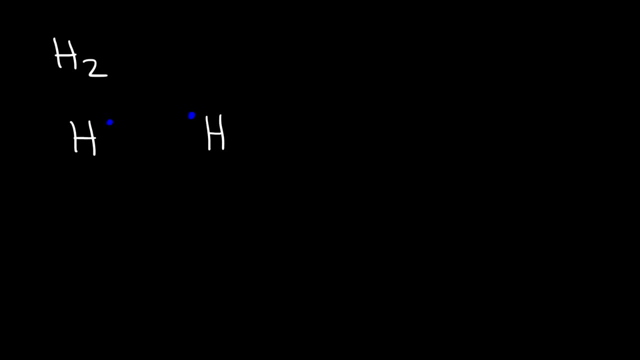 single valence. electron And hydrogen likes to form one single bond, So these two electrons will get together and form a single bond. So this is going to look like this: A single bond represents two electrons. So now let's look at another example. What about chlorine gas? Chlorine is the halogen which contains. 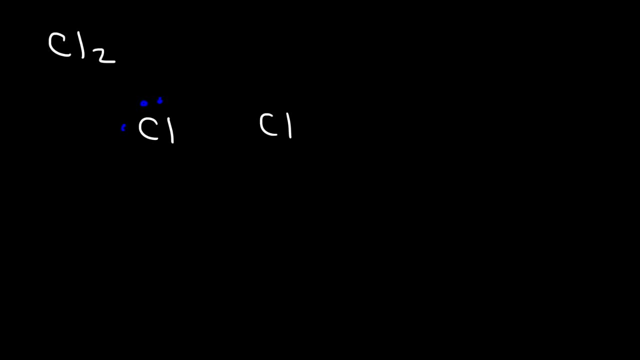 seven valence electrons. So if we draw the separated chlorine molecules, or atoms, it's going to look like this: Now the halogens, like fluorine, chlorine bromine, they form. they like to form only one bond, And so these two electrons will be. 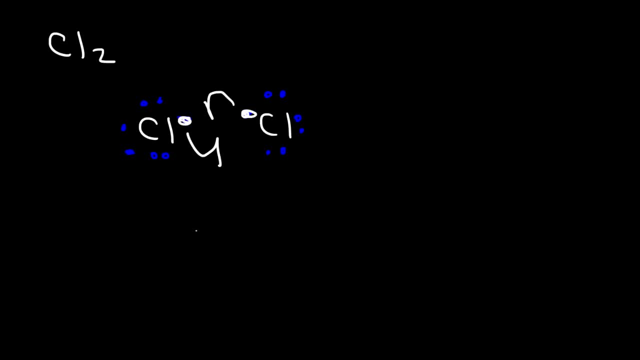 used to generate the single bond of the chlorine molecule. So this is how you draw the Lewis structure of Cl2.. So, as you can see, these two electrons were used to form the covalent bond within the chlorine molecule. Now it's very helpful to know the number of bonds. 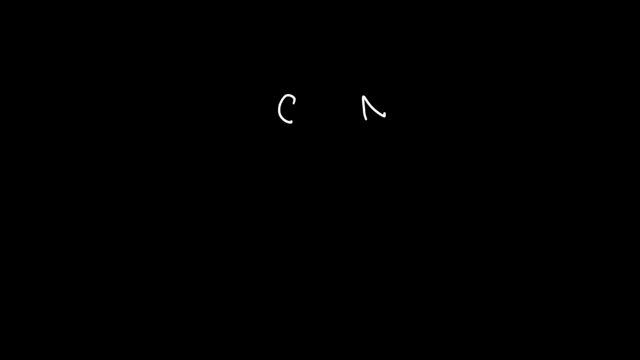 certain elements like to form. For instance, carbon has four valence electrons And in order to get eight, it likes to form four bonds. It forms a bond to acquire a new electron. Nitrogen has five valence electrons And in the 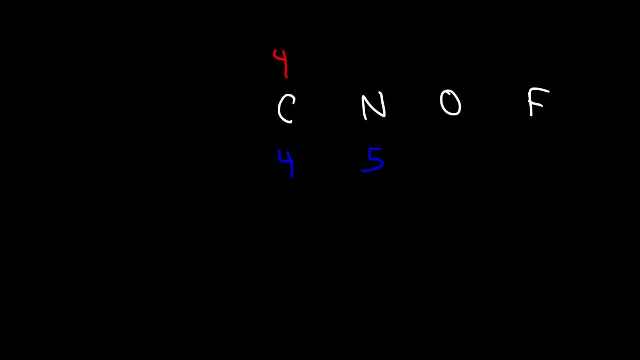 In order to satisfy the octet rule, it needs three more electrons to get to eight. so nitrogen likes to form three bonds to acquire those three electrons. Oxygen has six valence electrons. it needs two more to get to eight, and fluorine has. 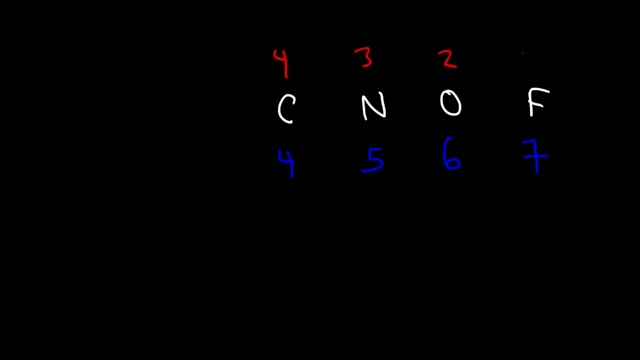 seven valence electrons and only needs one more to get to eight. So fluorine likes to form a single bond, oxygen likes to form double bonds. Now, to the left of carbon, you have elements like boron. Boron doesn't follow this nice trend. in fact, boron doesn't want to gain five electrons. 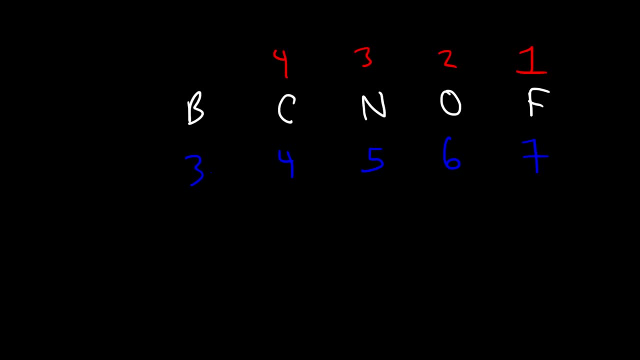 in order to satisfy its octet requirements. rather, it prefers to give away its three valence electrons, so boron likes to form two bonds. Beryllium prefers to give away its two valence electrons, so beryllium likes to form two. 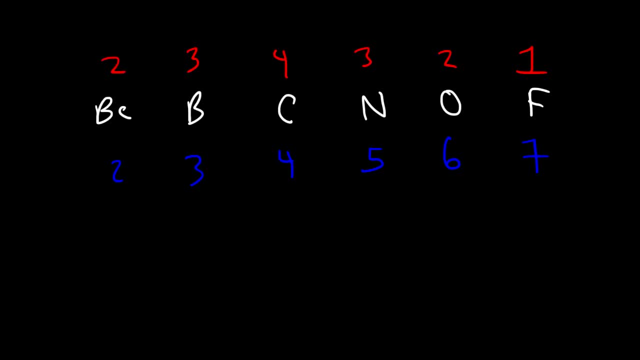 bonds. So elements on the right side of the periodic table, like carbon and everything to the right of that, they like to acquire electrons. So therefore you'll see that These numbers, they add up to eight Elements to the left of carbon, like beryllium and boron. they like to give up their electrons. 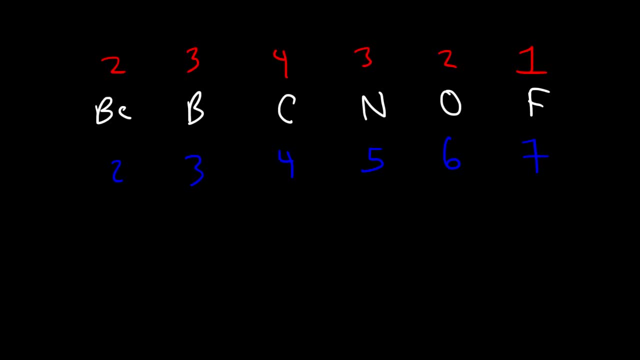 So the number of valence electrons tend to correspond to the number of bonds that they have or that they like to form. So that's the general trend that you see as you continue to draw Lewis structures in the future. So let's draw the Lewis structure of oxygen gas. 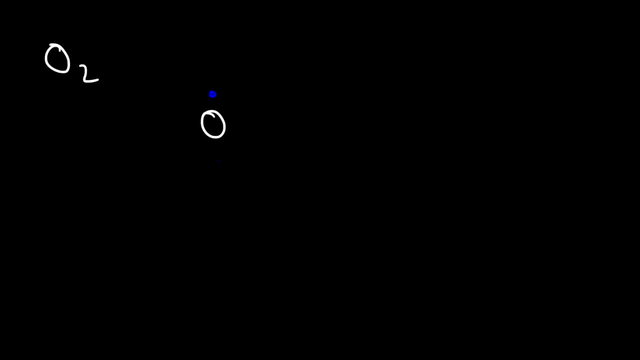 So each oxygen atom Contains six valence electrons, but I'm going to draw it like this. By the way, when I draw an arrow, a full arrow represents the flow of two electrons. a half arrow represents the flow of one electron. 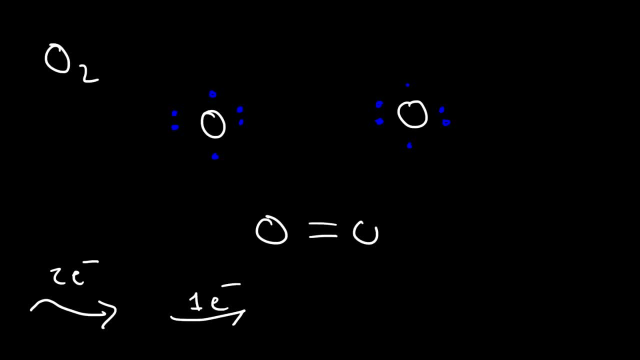 Now We know that Oxygen Is a double bond, So each bond represents two electrons, So therefore we need four electrons. These four electrons will be used to create this double bond, And so oxygen has four electrons left over that didn't participate in the reaction. 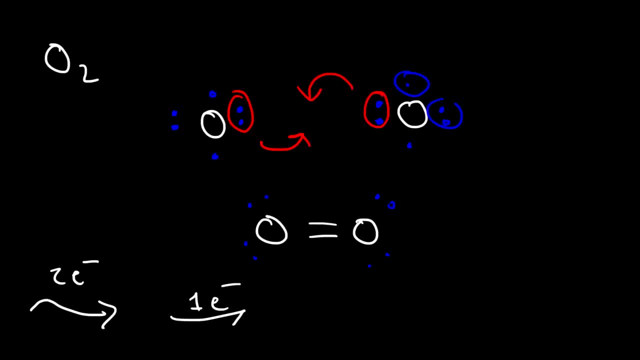 And on the right side we also have four electrons. So this is the Lewis structure Of the oxygen molecule. Now how can we draw the Lewis structure of methane using the same technique? So these cartridges, liksom teaspoonchez, And on the left side of theseın assumption to the two electrons, 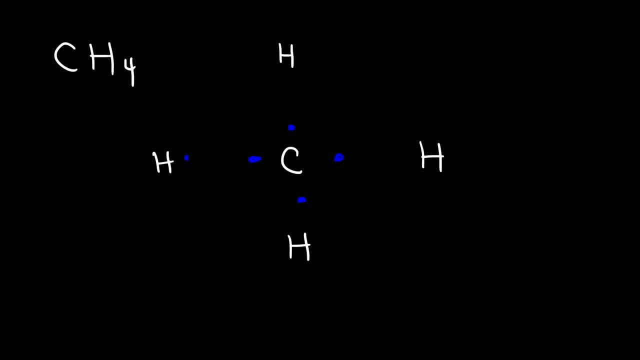 Carbon Honey. So when these elements get together to form methane, you can see that this is going to represent one single bond, this is another, and that's another single bond and here's another. So methane looks like this. This is the Lewis structure for CH4.. 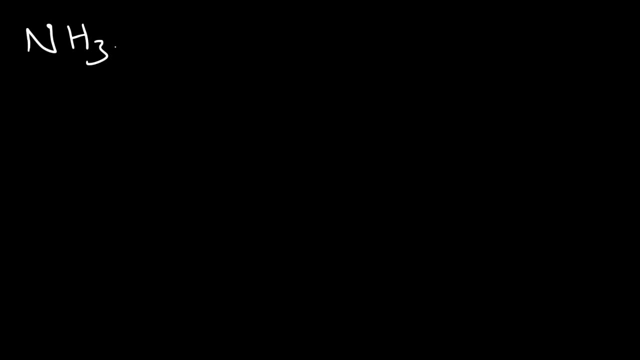 So let's consider our next example: ammonia. How can we draw the Lewis structure of ammonia? Now? nitrogen has five valence electrons, and hydrogen each contain one valence electron, So these two electrons will be used to form a single bond. that's another single bond. 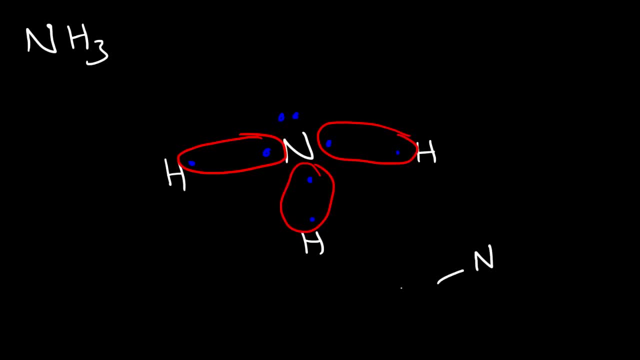 and that's going to be another single bond. So the Lewis structure for NH3 looks like this. Okay, As you can see, nitrogen likes to form three bonds, as you mentioned before, and hydrogen likes to form one, And in the last example we see that carbon has the four bonds that it likes to form. 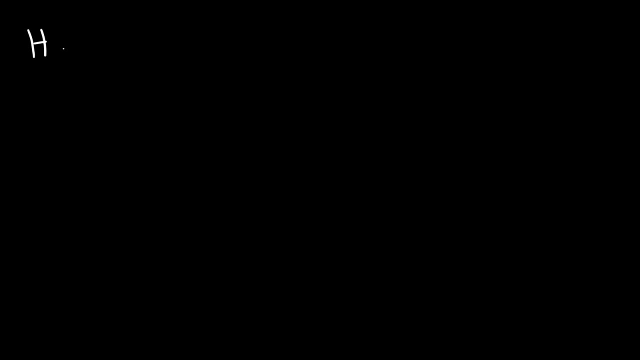 So now let's try another example. Let's draw the Lewis structure of water. Now, oxygen has six valence electrons, Okay, Okay, So we have a hydrogen electron. We can draw the Lewis structure of water with the help of a bit of paper, which I'm going. 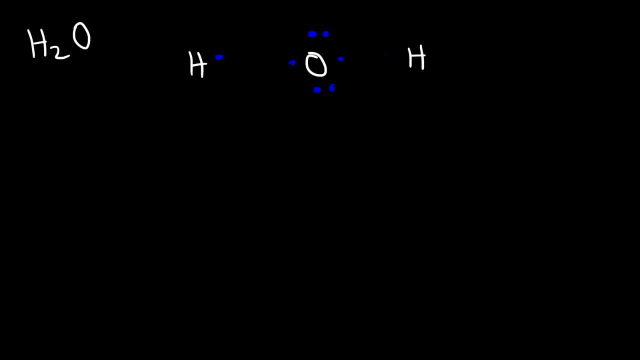 to place it like this. And each hydrogen atom only has one, So these two will be used to form a single bond and those two electrons will form a single bond. So you can draw the Lewis structure like this, but water does have a bench shape, so if you 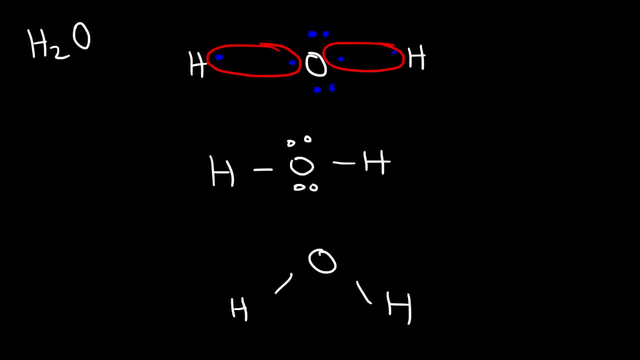 draw it with the appropriate geometry. technically it should look like this. So let's see how that works. Okay, so that's the lewis structure for water. it has a bent shape. now let's try another example. let's try oxygen difluoride. 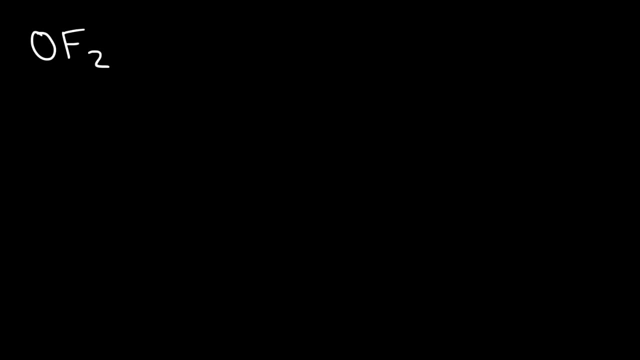 how can we draw the lewis structure for that? so oxygen has six valence electrons and fluorine has seven. now we know that fluorine likes to form a single bond and oxygen likes to form two bonds. so this is going to be one bond and there's the other. 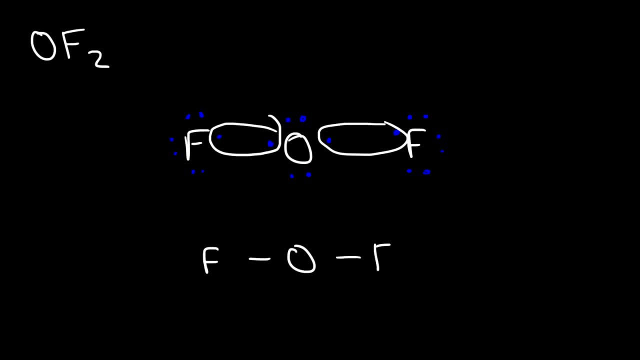 so the lewis structure looks like this. so that's the lewis structure of OF2, oxygen difluoride. but keep in mind, in reality it has a, a bent shape, just like water. now let's try a harder problem: draw the lewis structure for hydrazine. 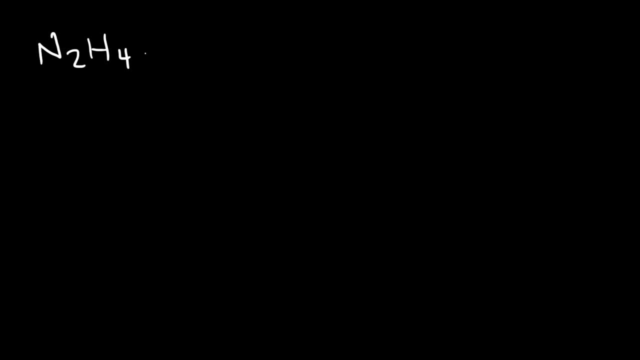 N2H2. now keep in mind: hydrogen likes to form a single bond and hydrogen likes to form three bonds. so because nitrogen likes to form more bonds than hydrogen, we're going to put it in the middle. so every nitrogen atom has five electrons, or valence electrons. 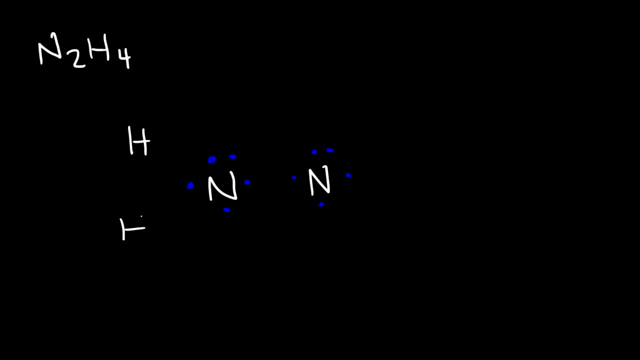 and the hydrogen atoms only contain one. so let's draw a lewis structure for hydrogen, N2H2 and fluorine likes to form two bonds, so we need to form three bonds with each or for each nitrogen atom, so we can say: this is going to be one bond. 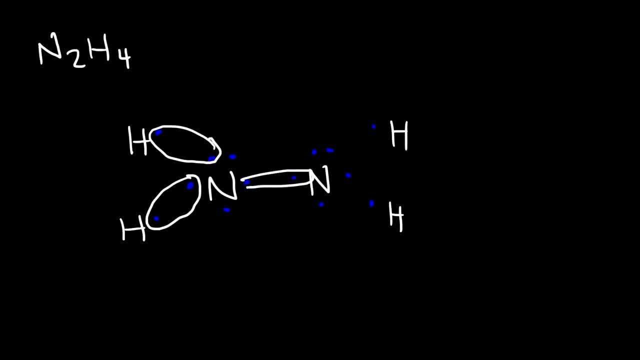 this is going to be the second bond here. that's the third bond, that's for the first nitrogen. these two could form a bond and those two could form a bond. so right now we have a structure that looks like this and, as we can see, that each nitrogen atom has two electrons left over, 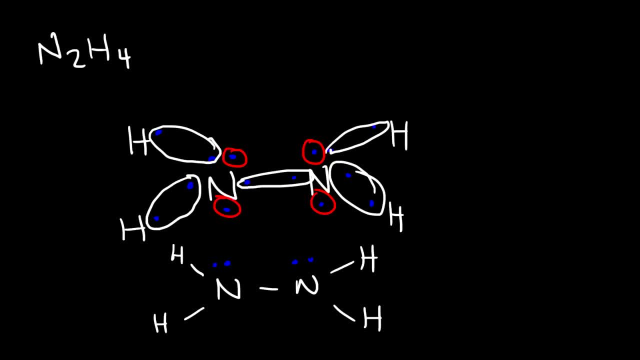 which we can draw as a lone pair. so that's the lewis structure of hydrazine N2H4. now let's try acetylene C2H2. so we have two carbon atoms and two hydrogen atoms. so every carbon atom has four valence electrons. 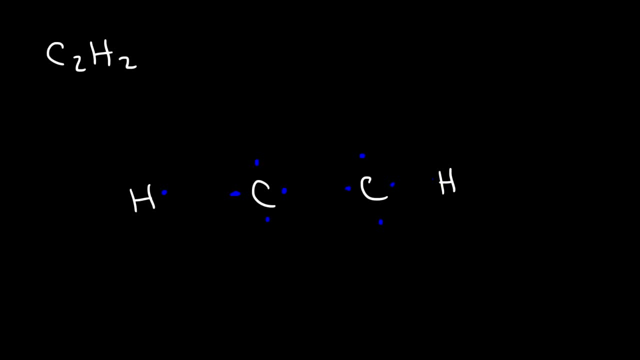 and hydrogen only has one. Now keep in mind: carbon likes to form four bonds and hydrogen can only form one bond, So this is the only bond that hydrogen can form. so we can draw that as CH and we could put a single bond between the two carbon.